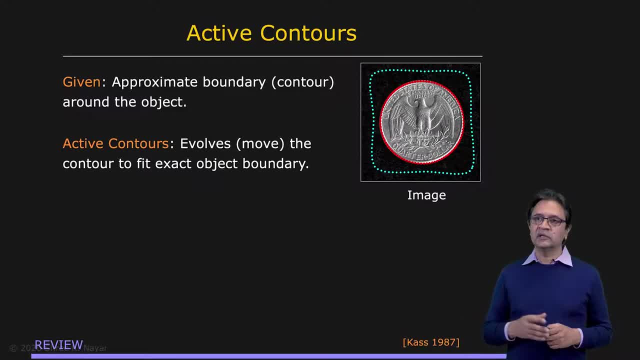 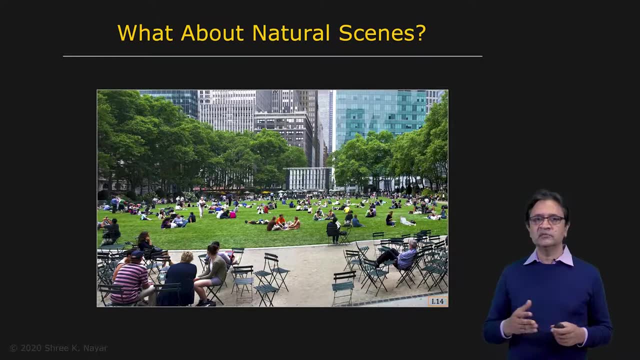 problem. in order to appreciate how hard segmentation is in general, one really needs to look at natural images. so the question here is: how does one segment this image into meaningful regions? for that matter, what is a meaningful segment in this case? if you look at, for instance, this man sitting in the front? 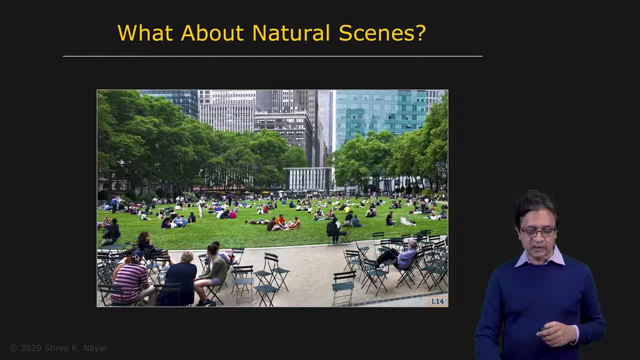 here is the cap that he is wearing, a part of him. does that- that's the cap plus the man- make a single segment, or are they to be treated as two different objects? it really depends on the task that you're trying to solve, the context itself. so we're going to 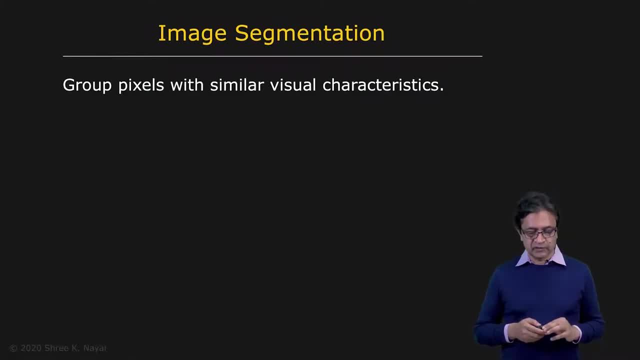 develop some very simple methods for image segmentation, and our approach is going to be to group pixels together in the image that have similar visual attributes of characteristics. so first we're going to start by looking at how we humans perform segmentation. what kind of rules, principles do we use to guide? 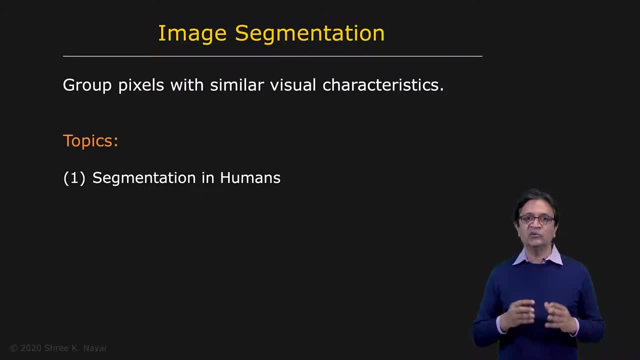 us during the process of segmentation. and what's really interesting here is that if you take a single natural image and you show it to two people and say: come up with meaningful segmentation, come up with the segments that are meaningful in these, in this image, you're going to get two. 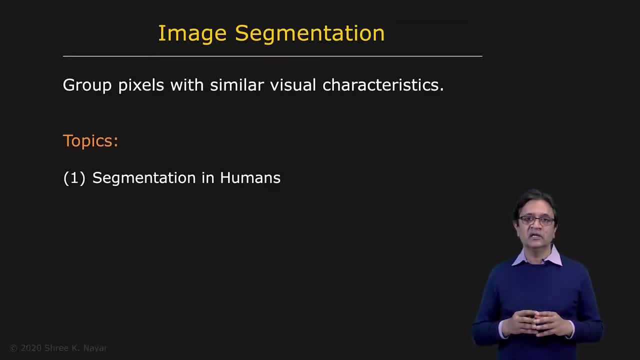 dramatically different results. in other words, segmentation is highly subjective for us, for humans, and that's because it's an ill-defined problem. so we're going to take a much simpler approach and simply say that segmentation is grouping together pixels that have similar visual attributes. in other words, we're going to treat it as a clustering problem at each pixel. 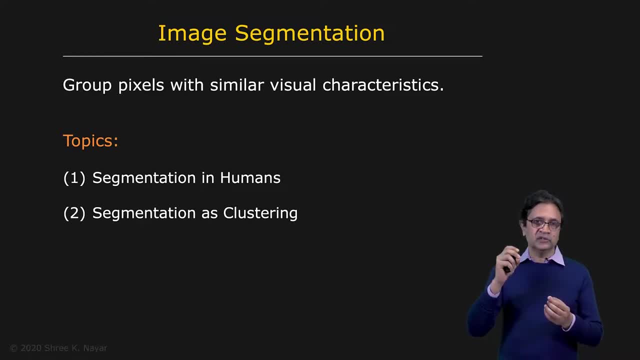 in the image, you have a feature vector which describes that pixel and that can be seen as a point in high dimensional feature space. in this feature space, we're going to cluster points together and those clusters are going to represent our segmentation, and that's why we're going to take a much simpler approach and simply say that 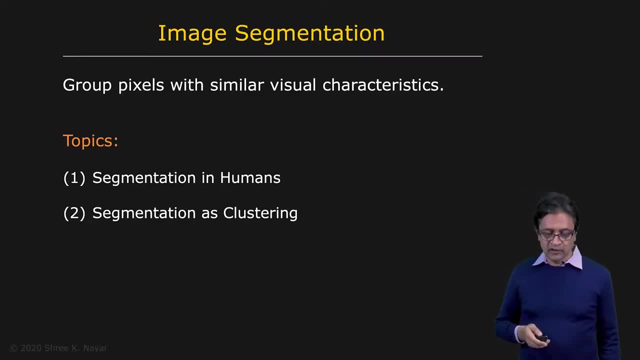 segments are meaningful regions or segments. so then at that point, really, the question is what clustering algorithm should be used. so the first algorithm we talk about is called k-means segmentation. so in this case, you specify the number of regions that you're looking for to be k.